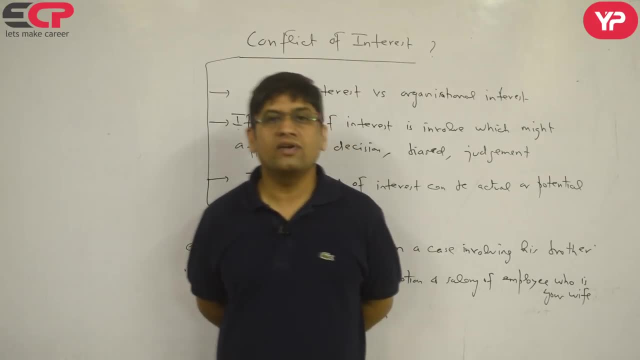 arise, Conflict of interest will arise. What is a conflict of interest? There are two terms in this: Conflict and interest. Interest means your self-interest and second is the requirement of the organization That, whatever decision you are taking, whether the direct or indirect, 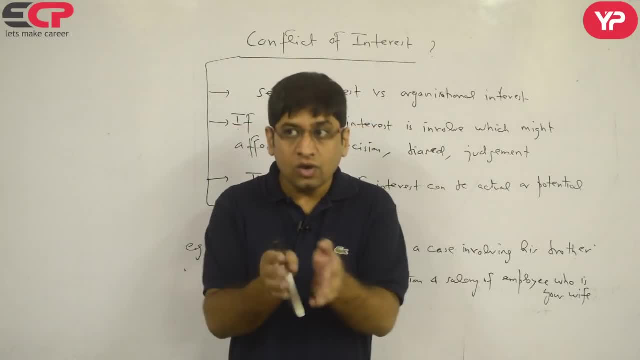 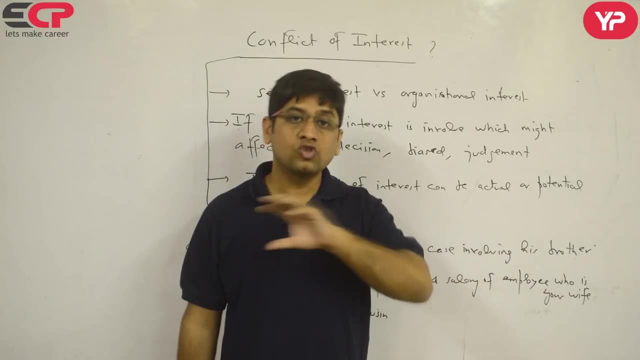 relation of that decision is with your interest or not? Are you related to somewhere, the decision which you are taking? Because whenever you sit on judgment or you decide as officer, then your decision should be totally fair and unbiased. That fairness and unbiased decision will arise only if you are not involved personally. 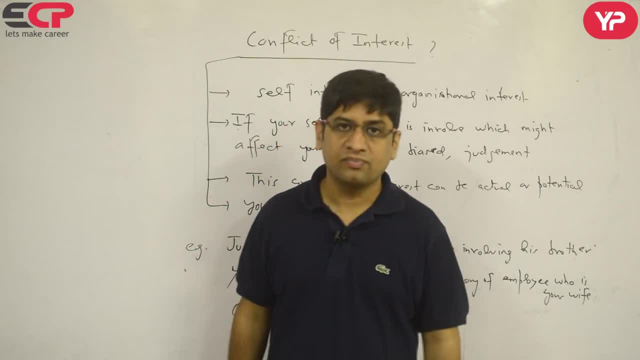 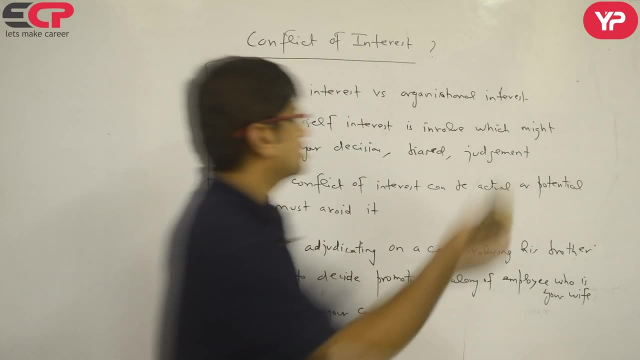 in that particular thing. You don't have any personal interest in it. What is a conflict of interest When the self-interest and the organization's interest, or I will say the organization's decision? there is some conflict between them. Organizational duty, which you 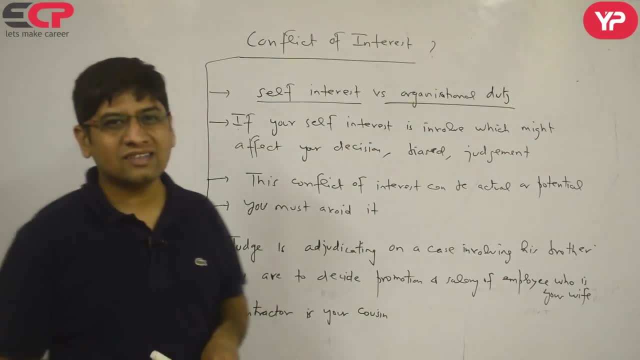 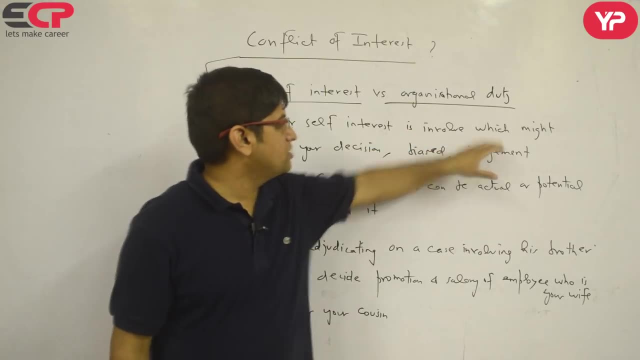 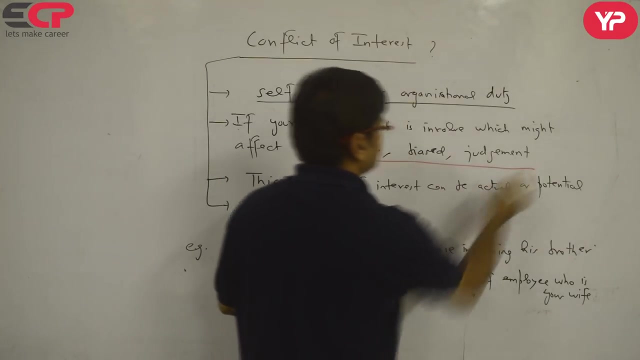 have to fulfill and your self-interest are somewhere overlapping Your interest is also the duty of the organization. If your self-interest is involved in which which might affect your decision, it may make your decision biased and it might affect your judgment Whether the decision which you are 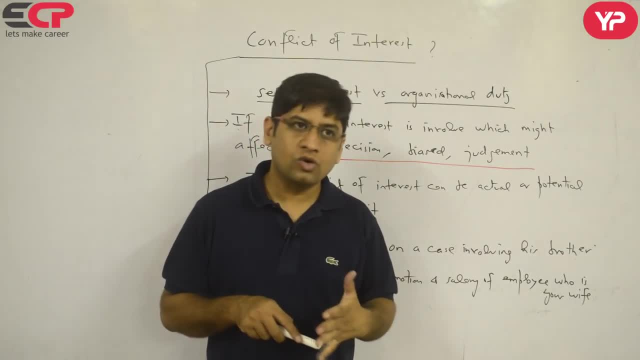 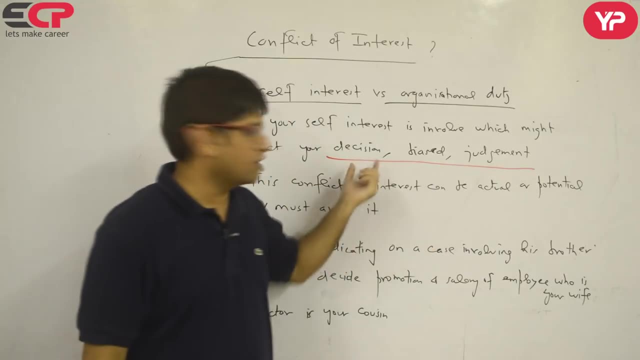 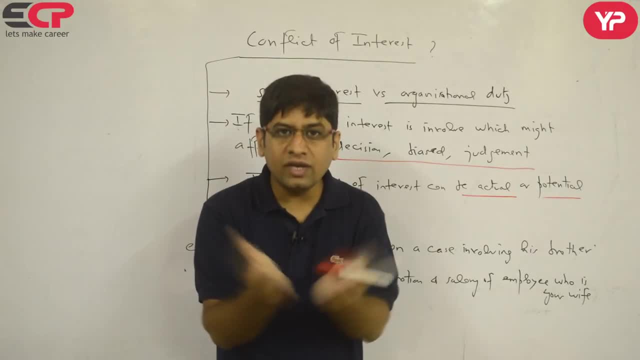 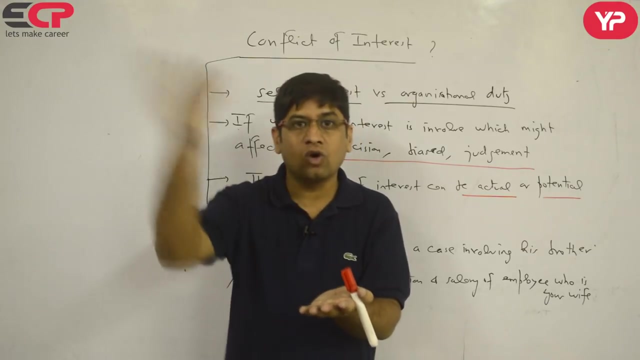 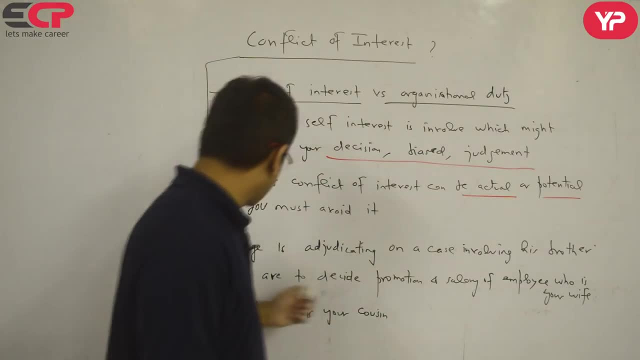 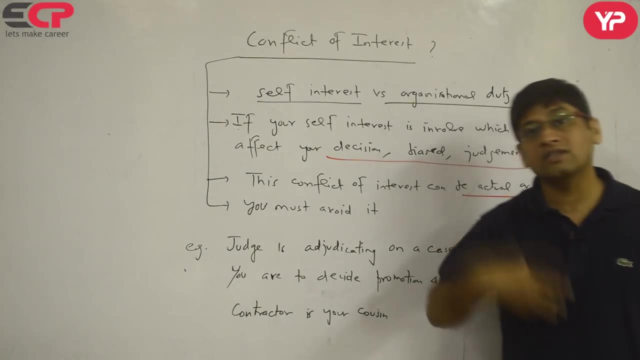